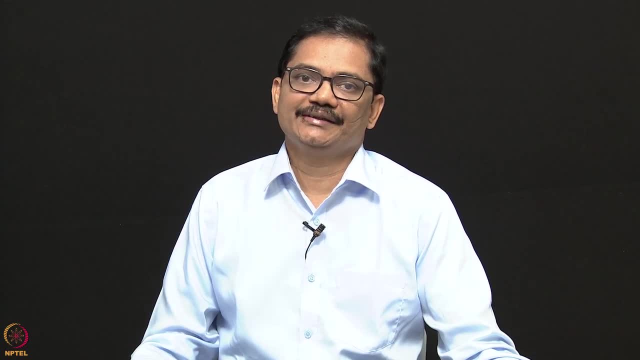 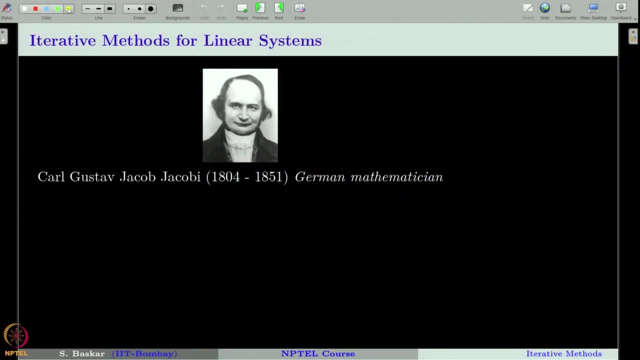 However, if you want only an approximate solution, then often iterative methods are good choice. In this lecture we will start our discussion on iterative methods. We will study the most simplest iterative method, called Jacobi method. This method is named after a German mathematician named Carl Gustav Jacob Jacobi. 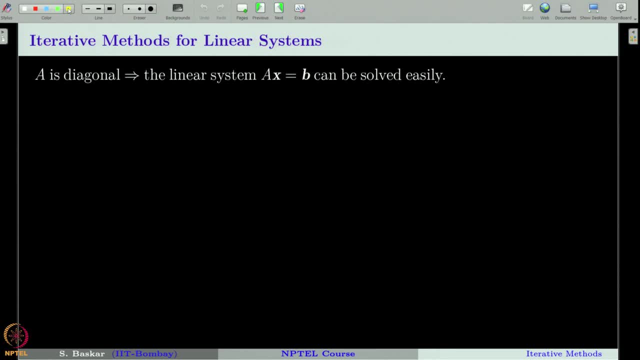 Well, if the given system is a diagonal system, then we all know that the linear system, AX equal to B, can be called a diagonal system. It can be solved very easily. We do not need to go for any elimination process, right? However, if the given system is not diagonal, then what to do? 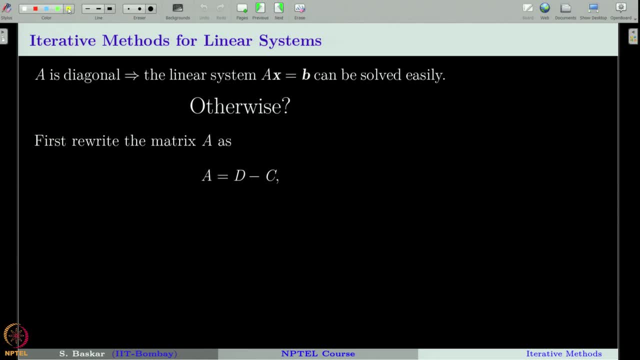 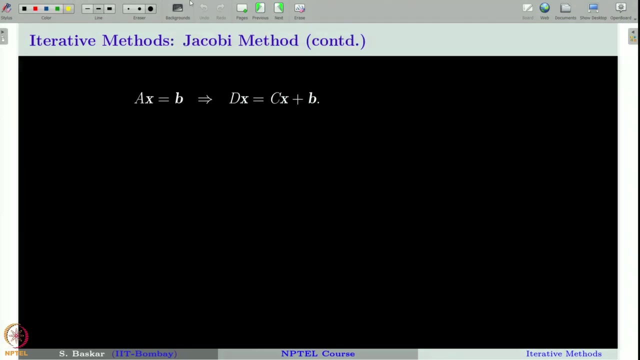 Jacobi suggests that you first write the coefficient matrix as D minus C, where D is the diagonal matrix whose diagonal elements are precisely the diagonal elements of the coefficient matrix A, and take minus C to be A minus D. Well, once you have written A in this form, you can write your linear system AX equal to B as D minus C into X equal to B, right. 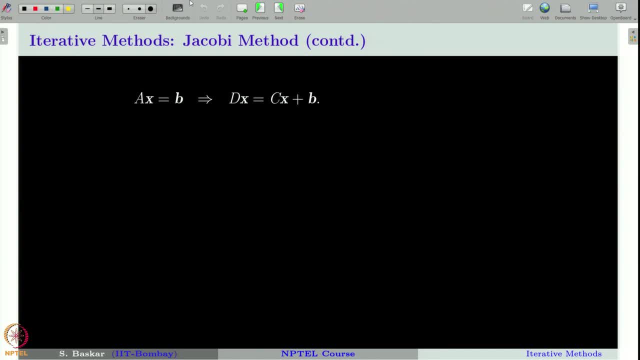 And that can be written as DX equal to B, And that can be written as DX equal to B, And that can be written as DX equal to B And that can be written as DX equal to CX plus B. Now you see, the left hand side involves only a diagonal matrix, but however, the system 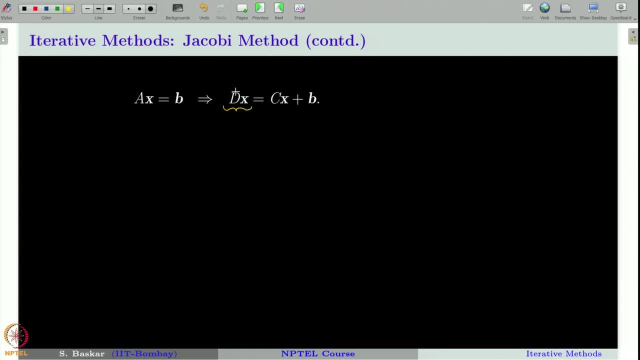 is not reduced to a diagonal system. Why? Because now the right hand side involves the unknown vector x right. Therefore, we have not gained anything by rewriting it. by rewriting our original system, A, x equal to b in this form, it is only that we have. 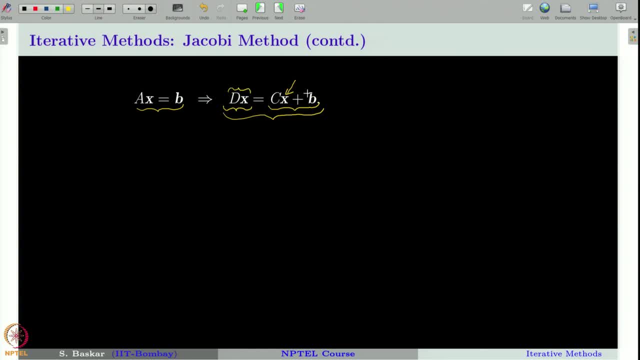 separated the diagonal elements on the left hand side and pushed all the other elements to the right hand side. Now just imagine that if this is somehow known to us, then the system will be reduced to a diagonal system. but there is no way that we can know this. 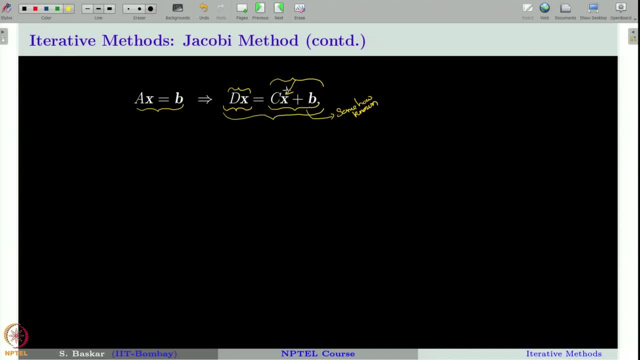 term, because knowing this is equivalent to knowing the exact solution itself. Therefore, the idea is: let us choose an arbitrary vector, say denoted by x, naught, and plug in that vector on the right hand side of this matrix expression. Then you see, this quantity is known to us, and thereby we can obtain a diagonal system. 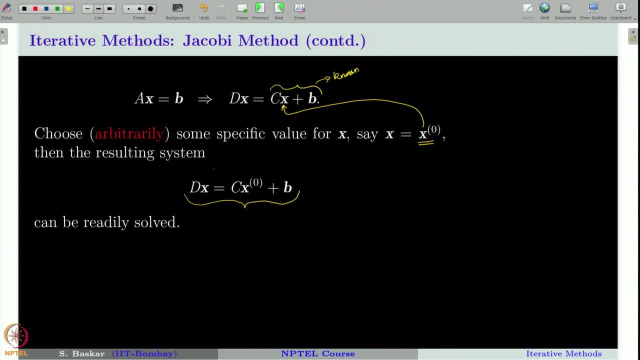 and this diagonal system can be readily solved to get a vector x. but note that this vector will not be the solution of our original system. Why? Because we have obtained it by plugging in. We have obtained an arbitrarily chosen vector. However, we can consider this as the first. 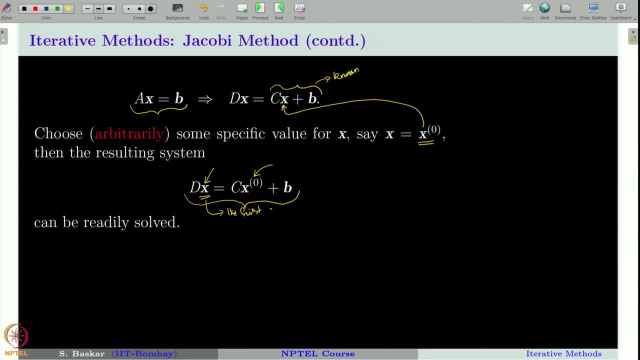 approximation to our solution x. We will call this vector as x 1, which is obtained by first choosing an arbitrary vector x. naught Again, we have this vector x 1, which is obtained by first choosing an error equation, which is obtained by first choosing an error equation. So this vector x 1 is the original. 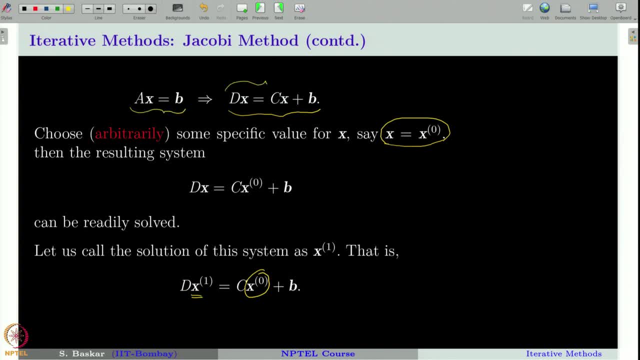 equation of the original system So we can put the 파이. we can go back to the previous equation, which was the original equation x 1 x 1 and plug in that on the right hand side of our equation. Remember, the exact solution of your original equation is the. 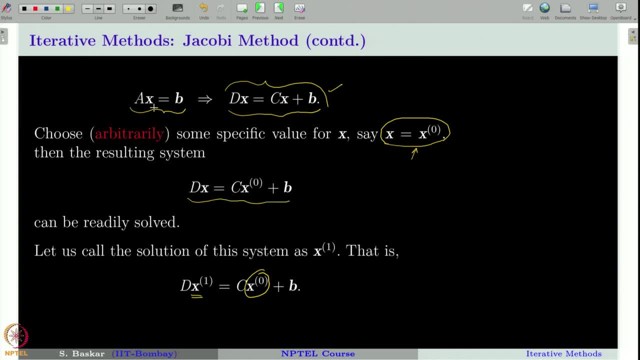 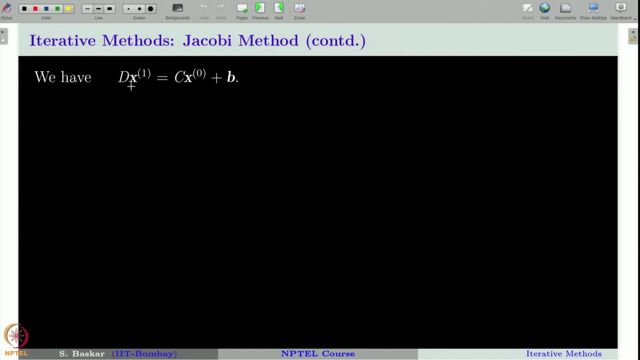 same as the exact solution of this equation. also, However, since we are plugging in some, we will consider it as a first approximation to our exact solution. that is the idea and that is called as x 1.. Once you obtain x 1 by solving this system, 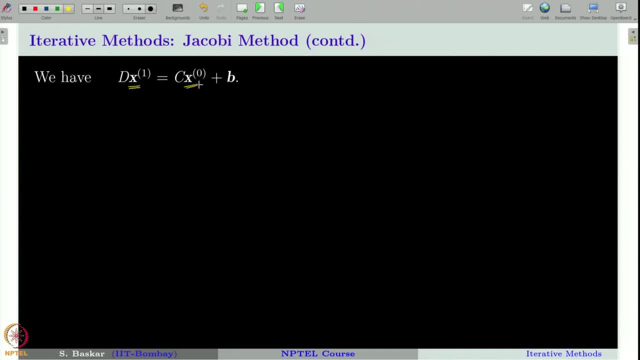 d x 1, equal to c x naught, which is known to as plus b. then you can plug in that x 1 on the right hand side expression. Now you see, instead of x naught, we are plugging in x 1 and solve this diagonal system once again and call the solution of that diagonal system. 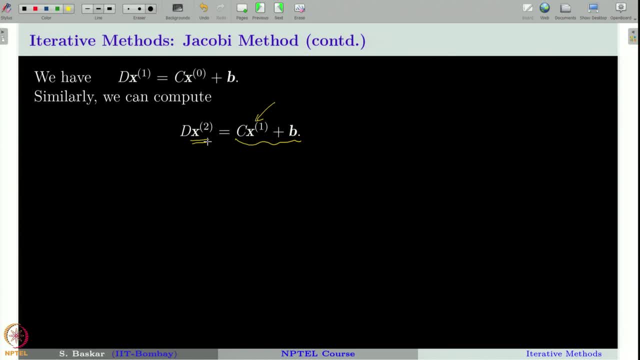 as x 2.. Once you get x 2, again plug in that vector x 2 into this right hand side expression and get x 3 and so on. In general, assume that you know this vector x 2.. x k for some, k equal to 0,, 1,, 2 or so on. For instance, if k is equal to 0, we have chosen. 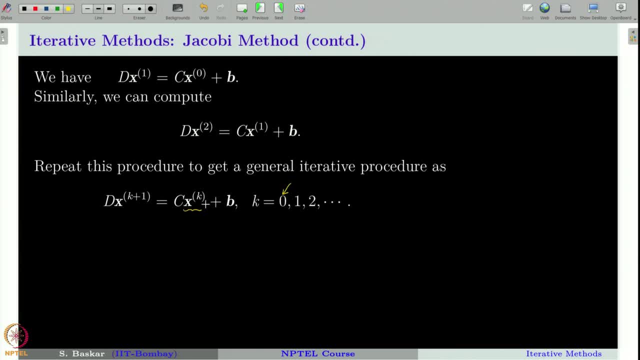 this vector, which is x, naught arbitrarily right, and then we got x 1 and by taking k equal to 1, you plug in x 1 on the right hand side, get x 2 and so on. In general, at the k th level you have obtained the vector x k and when you go to the k plus 1 th level, 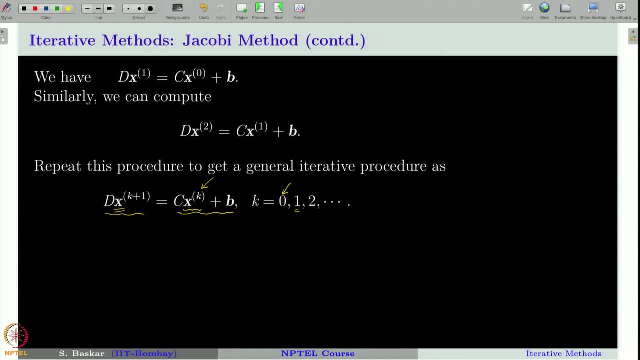 you plug in that vector x- k on this right hand side expression and solve this diagonal system to get the vector x k plus 1.. In that way you are generating a sequence, x naught which is arbitrarily chosen. then you are getting x 1 from the vector x k plus 1.. 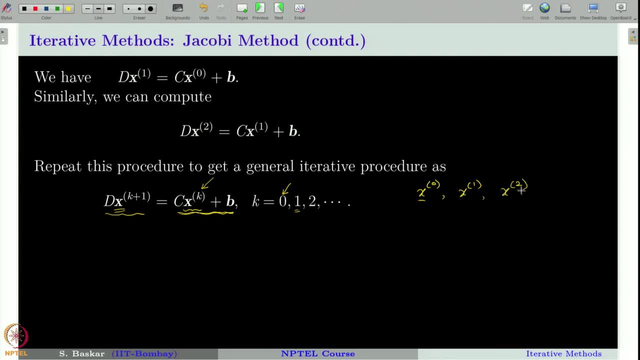 From there, then, plugging in x 1, you are getting x 2 and so on, So you are getting a sequence of vectors like this, and this process is called the iterative process, or iterative procedure means what you start with, the x naught, and you have an expression say: let us denote it. 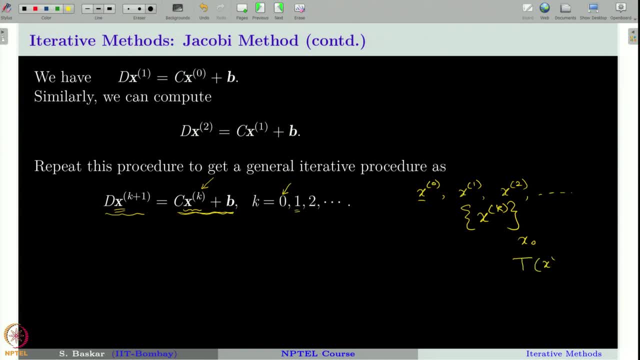 by T of x, So it is an expression involving a vector x. in that expression you are plugging in x naught. let us call this as x naught, right? you plug in that x naught, get x 1. and again plug in x 1 into this expression: get x 2 and. 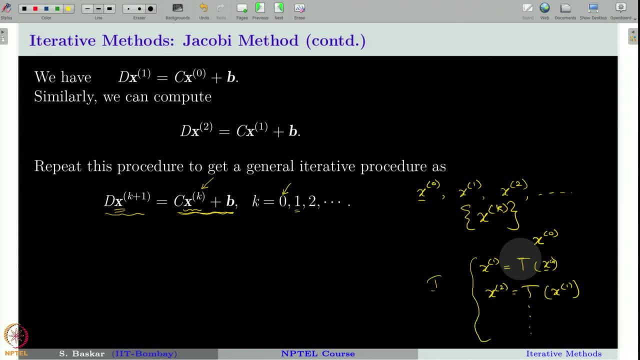 so on. So this procedure is called the iterative procedure. So if you want to plot a invertible matrix, then you can write this expression rather in a nice way like this: by multiplying both sides by D inverse, and in that way we get: 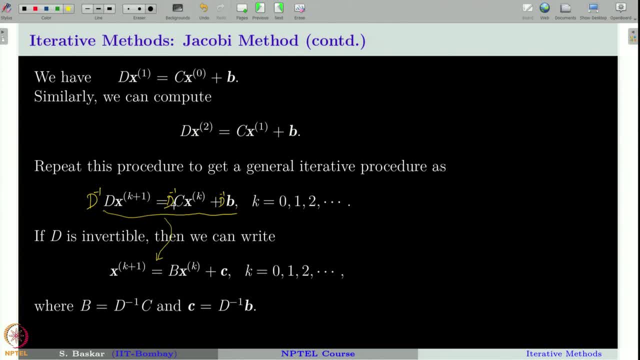 x k plus 1, equal to D, inverse into C, which we will denote by B, into x k plus the vector C, which is nothing but D inverse B. So this is a iterative procedure that leads to a sequence x- k, which is called 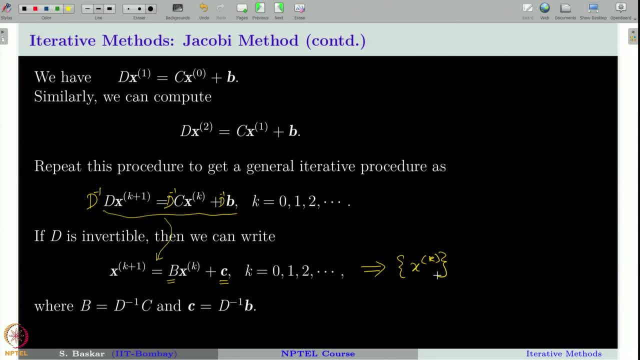 the iterative sequence, and this method of generating the iterative sequence is called the Jacobi method. In general, an iterative method is that for which we have a sequence generated in this form, where the function t is something given to us. Different form of t will lead to different methods. In particular, in Jacobi method, the function that is called 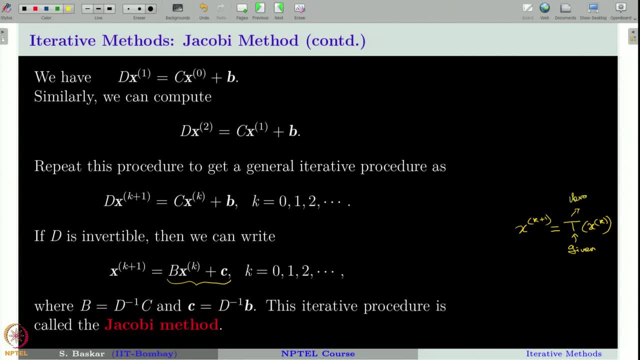 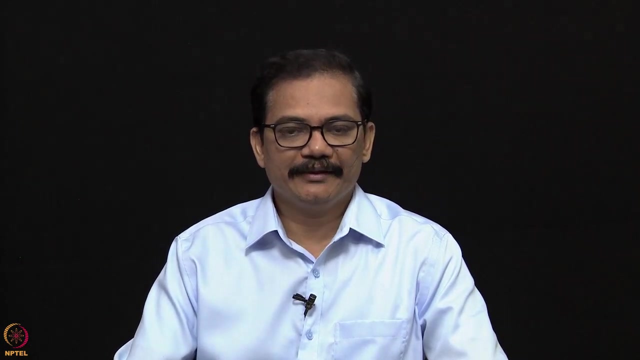 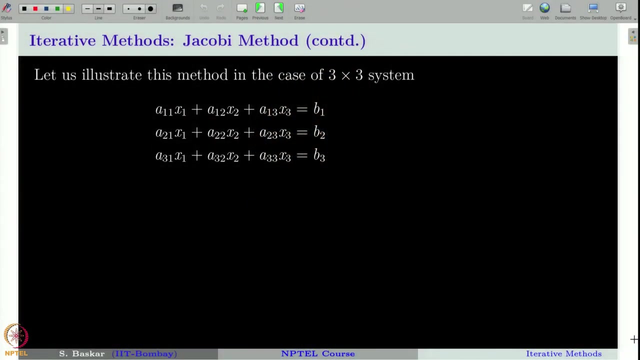 the iterative function and that t in the Jacobi method is given by this expression. I hope we have understood the Jacobi method. Let us try to understand the Jacobi method in a rather simple way by looking at each equation of the system separately. What we did so far is the Jacobi method in the matrix. 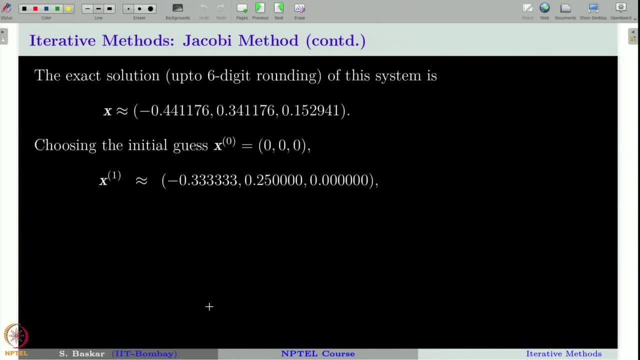 we got in our first iteration. It is minus 1 by 3 and this is 1 by 4 and 0. So this is 1 by 3.. The next step is to get x 2.. How do you get it? You plug in vector x 1 on the right hand. 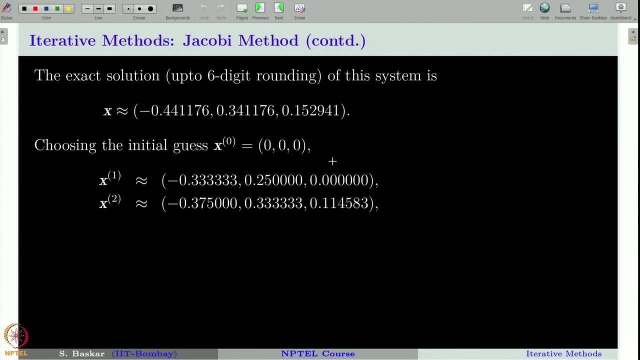 side of the Jacobi iterative formula and get x 2.. Once you get x 2, again, plug in x 2 on the right hand side to get x 3.. Once you get x 3, plug in on the right hand side of the. iterative procedure: Get x 4.. Remember x 3 is in the rocks. you are able to see the overWhich isuri: x, Therefore x 2. How you find that X 3 is einmal squared over x 2 and x 2 is plus star, or c 1 over x 2 plus t. Enter in: the decoding. So next step is to plug in x 2 to x 1, x 1 over x 2 to get x 3.. Now the vector x 1 on the right one side of the€. collisions, offensive1, väldigt, preparations and the. 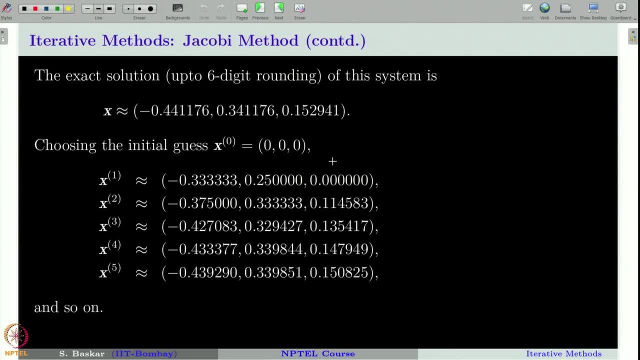 4, once you get x 4 you plug in on the right hand side to get x 5 and so on. So mathematically this process will go on infinitely and generates a infinite sequence: x, k, right. but on a computer you cannot go on doing this process. we have to stop this process at some point we will. 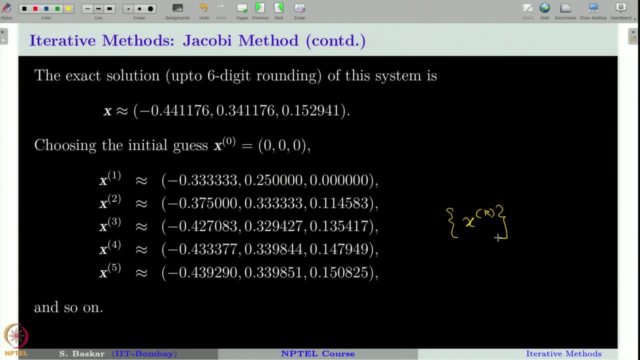 see later how to stop this procedure, but in this example I have stopped my computation at the fifth iteration. Now let us observe coordinate wise: in the first coordinate we got minus 0.3333, in the second one we got this value: third, fourth, fifth, just compare. 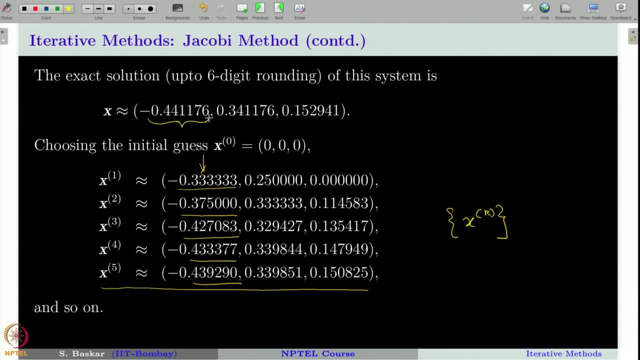 it with the value That we are supposed to get, at least up to six significant digits. we are supposed to get this value and when you see the first coordinate of the iterative vectors, you can see that we are going closer and closer to what we want as we go on computing the iterations. 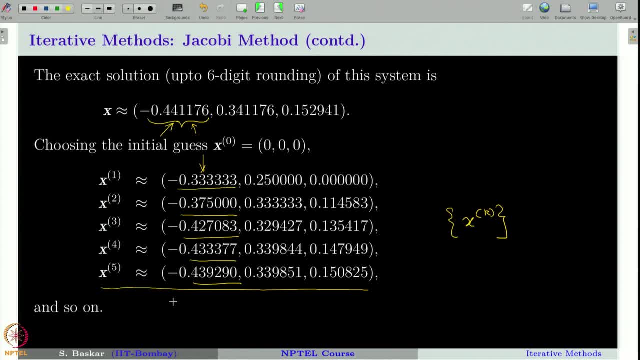 That is what we meant by saying that we seems to be converging to the expression. The same situation is also happening with the second and the third coordinate. you can clearly observe that as we go on with computing the iterative sequence, the coordinates are going closer and closer to the corresponding coordinate of the exact solution. So it seems. 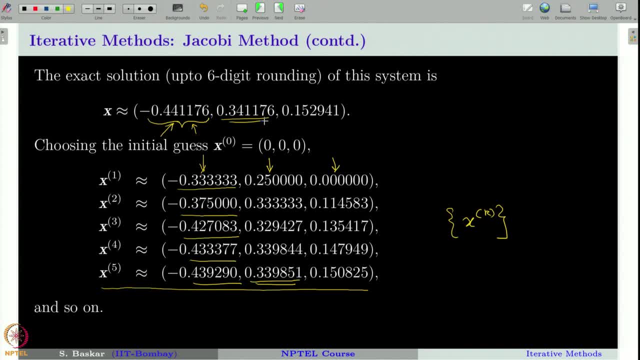 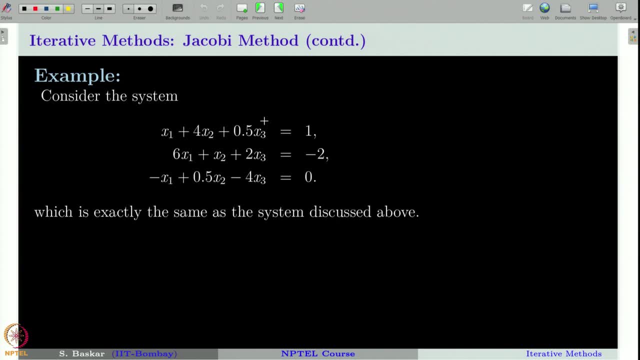 that the Jacobi method is correct. It is converging for this system and for the initial guess that we have taken. Next we will go to another system. you can see that in this system we have just interchanged the first equation by the second equation of our previous system and the second equation 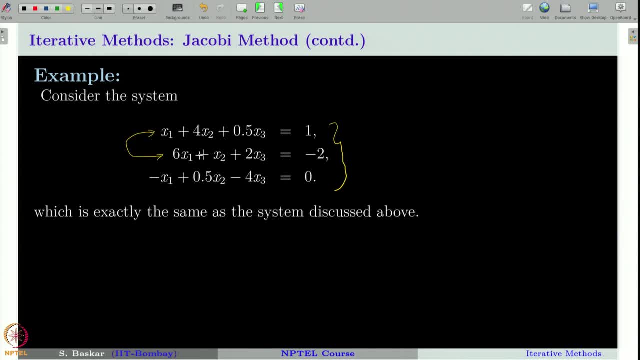 is taken as the first equation of our system. In that way, we have not changed the system mathematically, because we have only interchanged the first and second equation. Therefore, the exact solution of the previous system is the same as the exact solution of the present system. 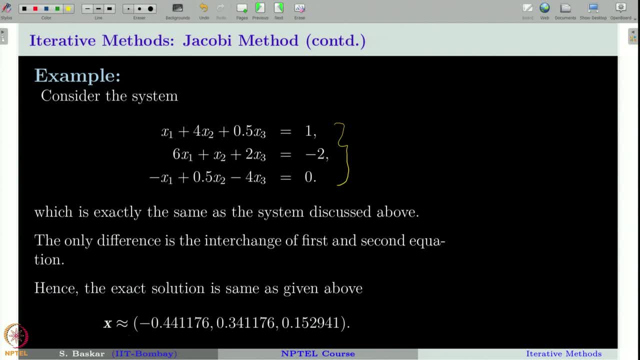 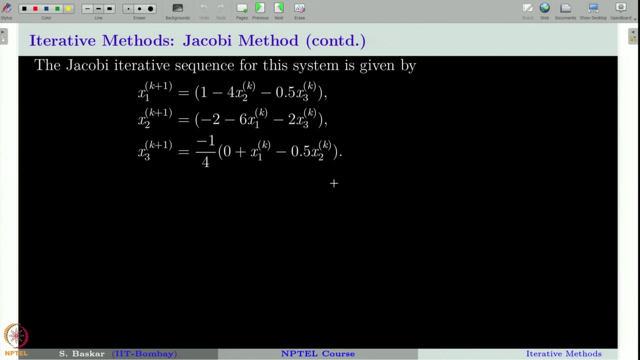 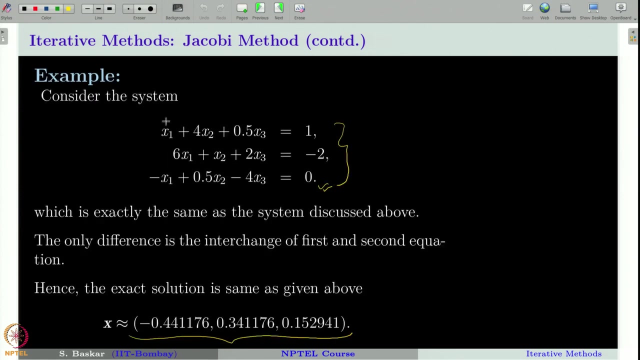 If you recall, the exact solution is this: Given like this, up to 6 significant digits, Now let us write the Jacobi iterative procedure for this system and see numerically whether that sequence is going to converge or not. So when you go to write the Jacobi iteration for this system, you can see that the diagonal 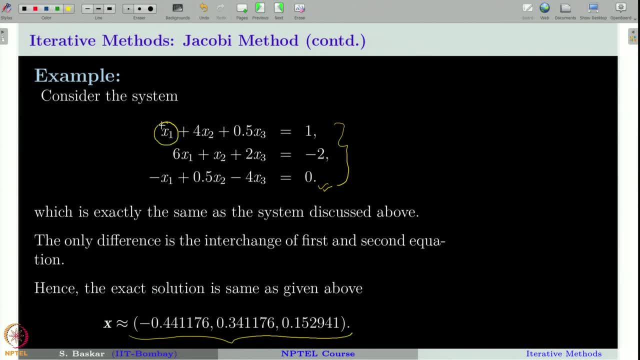 element Now for the first term is this: If you recall, for the previous system, the diagonal element for the first equation is this, because that was sitting as the first equation. Now the diagonal element is this and similarly the diagonal element of the second equation: 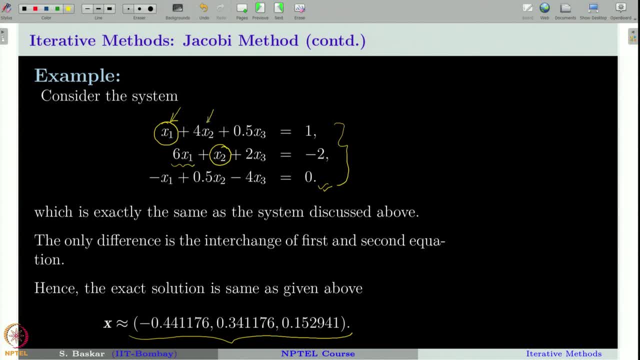 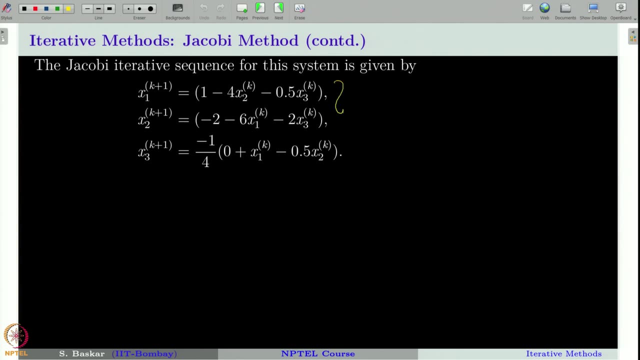 is also changed. Previously this was the diagonal element, now it is changed to this one because we have interchanged the equations and therefore now we have a different expression for the Jacobi iteration. If you recall, the system is same mathematically but the Jacobi iteration is different because 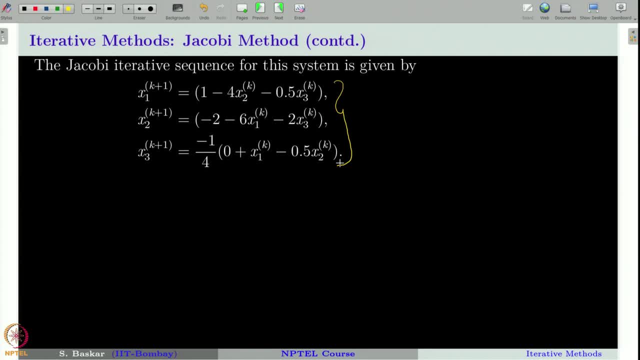 the equations, positions are changed. Let us go to compute the iterations. for that we need an initial guess. Again, I will choose 0 vector as my initial guess. with that, my first iteration, that is x, 1 is given by 1 minus 2 and 0, that is very clear. 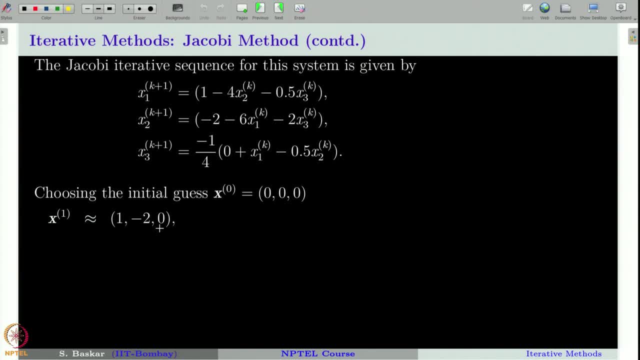 Now I will plug in x 1 on the right hand side of this expression and then get x 2, and that is given by this vector. Now I will plug in x 1 on the right hand side of this expression and then get x 2, and. 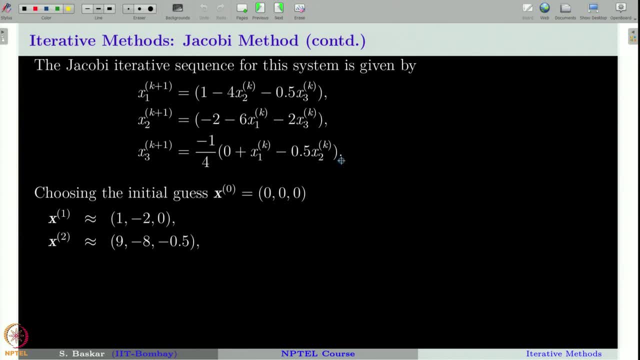 that is given by this vector. Now, once you get x 2, plug in on the right hand side, get x 3, plug in x 3 on the right hand side, get x 4, and so on. Observe the coordinates. 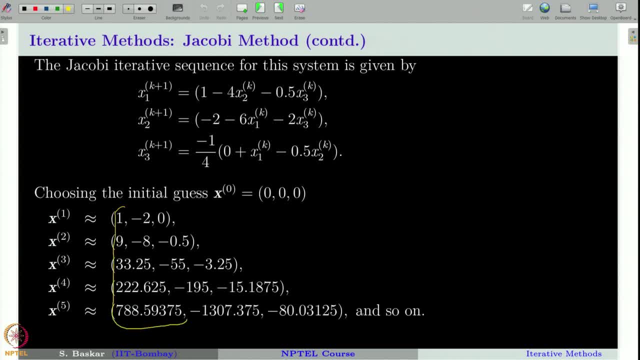 You started with 1, that became 9 in the second iteration. further it became 33 in the third iteration, and 2,, 2,, 2 and so on. So that gives us a feeling That iteration is going away from the exact value. The same situation is happening in the second. 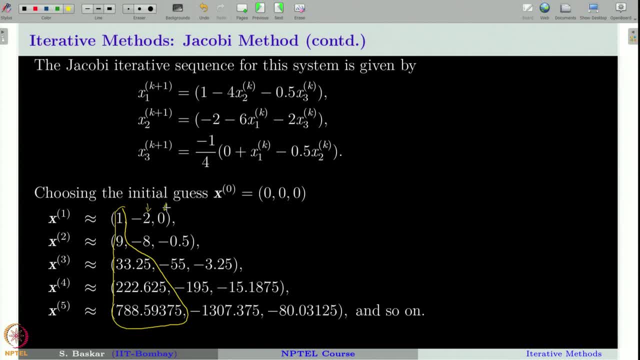 coordinate as well as in the third coordinate also, That clearly shows us that we are going away from the exact solution and gives us a feeling that the Jacobi iterative sequence for this system, when we started with the initial guess as the zero vector, is going.